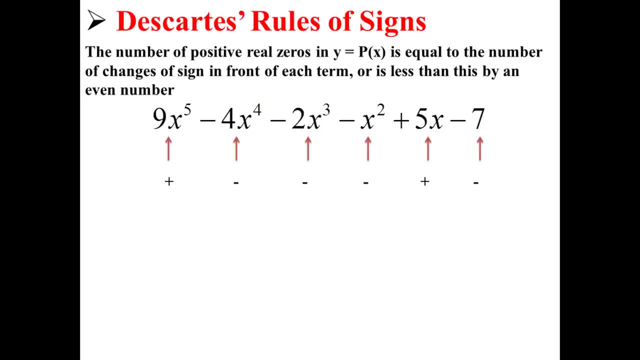 It goes from positive to negative to negative to negative to positive to negative. So we have three changes: From positive to negative, from negative to positive and then back from positive to negative. So we either have three positive real zeros or one positive real zero. 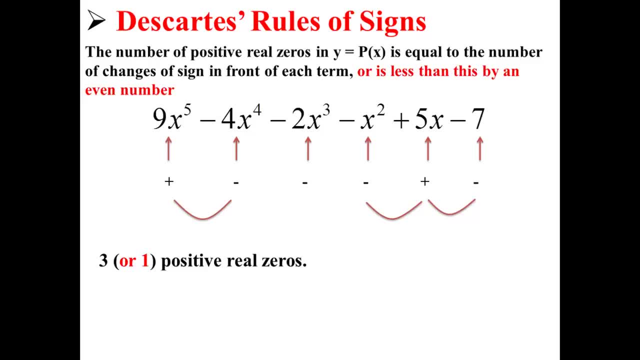 Because it is less than 3 by an even number, in this case 2.. So three or one positive real zeros. Next, the number of negative real zeros is the same as the number of changes of sign in front of the terms of p of negative x. 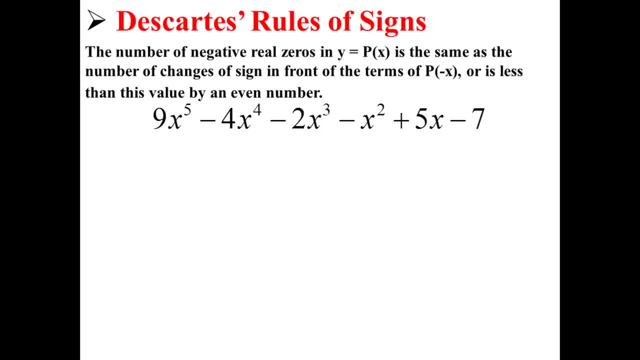 or is less than this value by an even number. So here we have p of x. We need to rewrite this equation as p of negative x. So we have 9, negative x to the fifth minus 4, negative x to the fourth minus 2, negative x to the third. 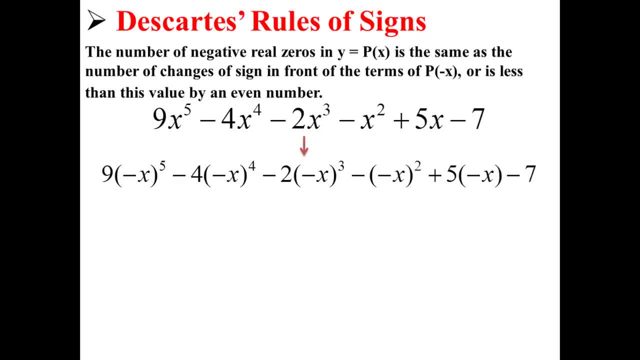 minus negative x to the second, plus 5 times negative x minus 7.. Which simplifies further: to negative, 9x to the fifth, minus 4x to the fourth, plus 2x to the third, minus x squared, minus 5x minus 7.. 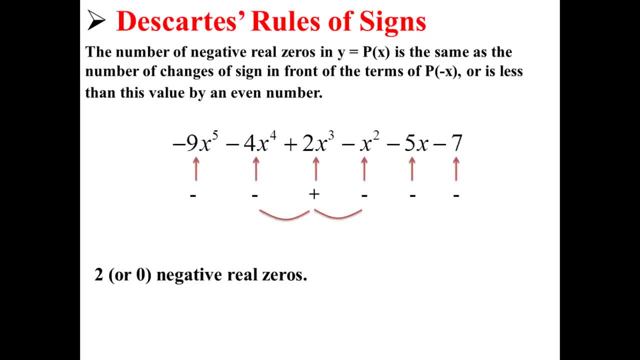 Now we look at the sign changes of this equation. Here we have two sign changes, From negative to positive and positive to negative. That means we have either 2 or 0. Or 1, negative, 0, 0, 0, 0.. 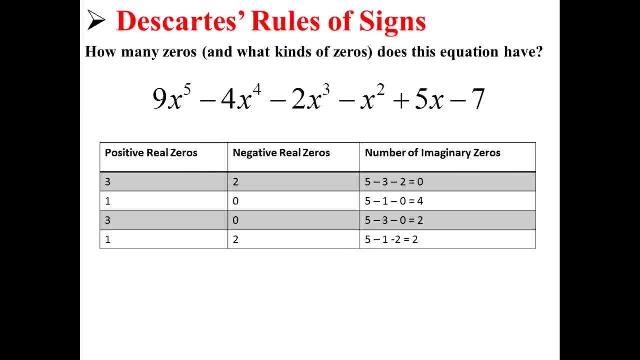 Before negative real zeros. Here are all the different possibilities. We could have three positive real zeros, Two negative real zeros And zero imaginary zeros. Or we could have one positive real zero, zero negative real zeros and four imaginary zeros. 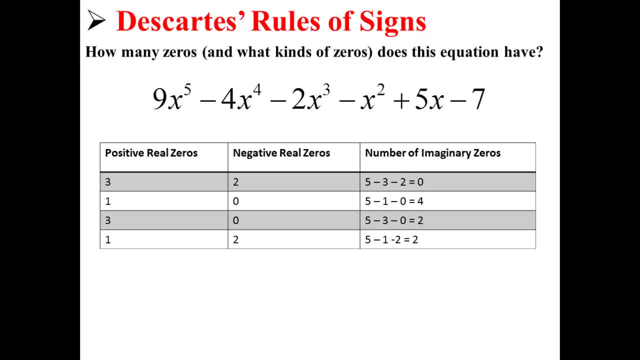 We could have three positive real zeros, zero negative real zeros and two imaginary zeros. real zero, two negative real zeros and two imaginary zeros. This is according to Descartes' Rule of Sines.